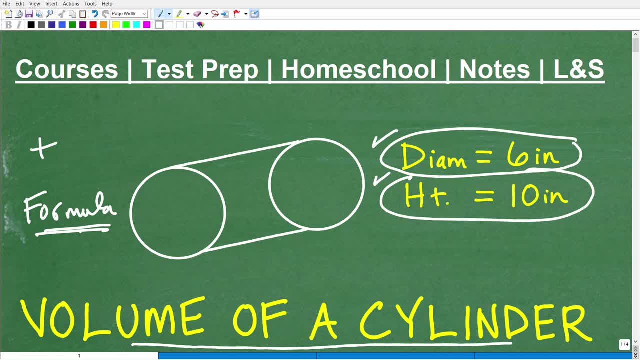 maybe one formula that I would say: yeah, you know, if you forgot that, that's fine, But something when you're dealing with like spheres or cylinders, I would suggest that you want to try to put this into your long term memory. Anyways, I'm going to show you the formula to this and the correct answer in just one second. But if you think you can do this problem, go ahead and put your answer into the comment section. I'm going to show you the correct answer in just one second, Then I'm going to show you the formula And then we're going to walk through how easy it is to find the volume of a cylinder. But before we 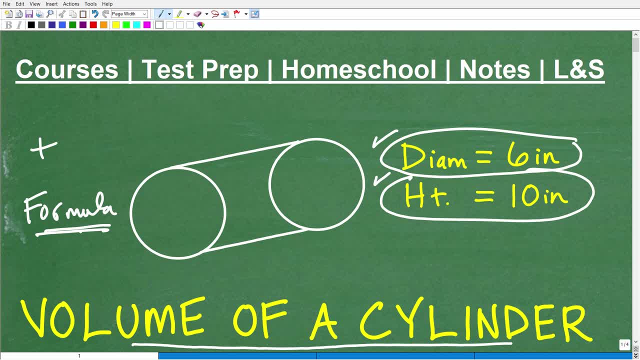 get going. let me quickly introduce myself. My name is john. I'm the founder of TC math Academy. I'm also a middle and high school math teacher. I have been teaching math for decades. really is my true calling to help as many people as I possibly can learn mathematics. I'm going to tell you right now, all of you could be successful math, And I'm especially speaking to those of you that struggle in math. okay, the really the most important thing you need is to learn from someone you actually understand, or whatever you're learning from. maybe you're learning you know using 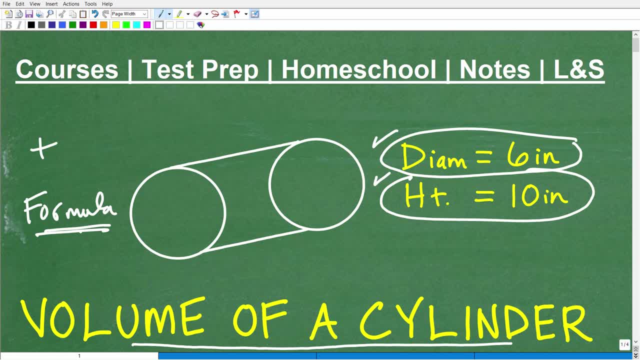 some sort of video program or software or reading some sort of book. But if you're not understanding what's going on, you're going to be kind of wasting your time trying to figure out. you know, you know mathematical concepts and principles, right? So math is a technical subject And the way I like to teach math is in an easy to understand, simple way. So anyone and everyone can get this stuff without watering down what you need to know. So if you need help in your current math course or maybe some sort of special test that you're getting ready for something, 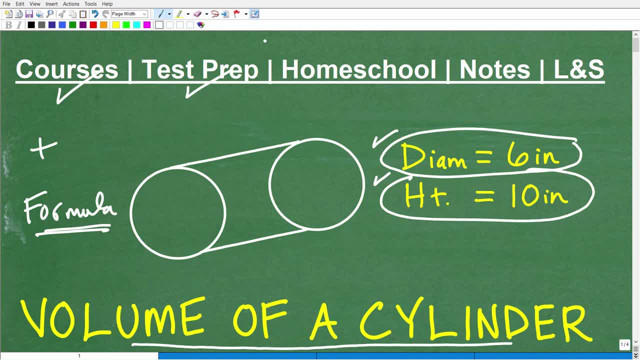 that has math on it, things like the GED, SAT, maybe a teacher certification exam, or, if you're homeschooling mathematics, check out my math help program. I'm going to leave a link to it in the description of this video. I literally have over 100 plus different math courses that span these categories and much, much more. I'm also going to leave links to my math notes in the description as well. You absolutely need a great pair of notes to study from Now. hopefully, you're taking your own awesome notes, But if you don't have great notes right now, you need to improve those things. 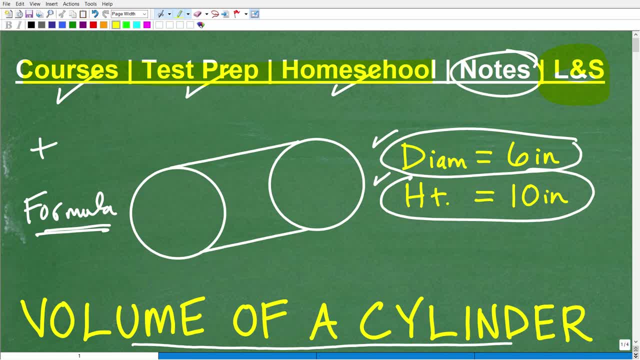 But in the meantime, you could use my notes if you like, And if this video helps you out, don't forget to like and subscribe, as that definitely helps me out. Okay, so let's go ahead and take a look at the volume of this cylinder. Again, the diameter of the cylinder. So let's give you a little bit of a hint here. The diameter is the width of this part right, Here's a circle and this is a circle. Matter of fact, let me just go ahead and define what a cylinder is. We got a circle here and a circle here. A cylinder would be like a can, right, Some sort of can. 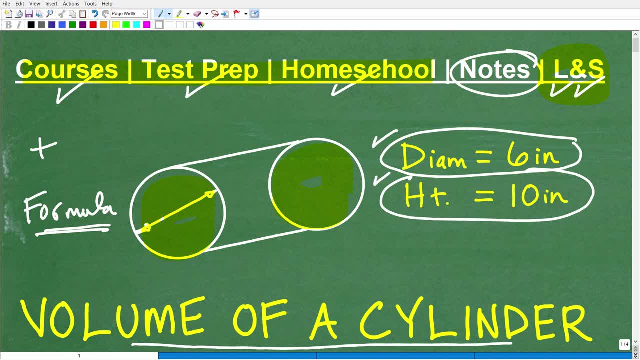 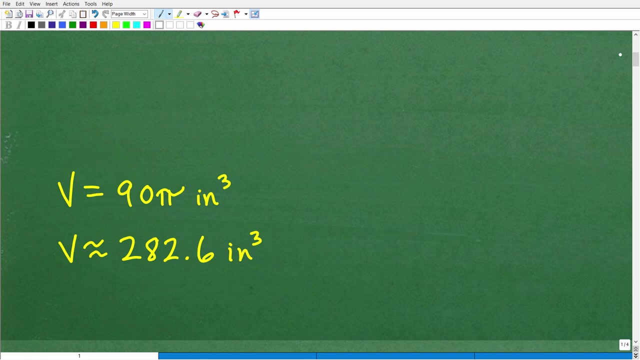 Like a can of soup, soda can, something like that. So the width of the circle, okay, these end caps, if you will, the top or bottom of it, the width of it is the diameter, Okay, so that's what that is, And then the height here would be the length. That's this dimension, right there. But let's go ahead and take a look at the answer. So here it is the volume of the cylinder, the exact volume, Okay, and you can see, here I'm using two different symbols. Here I'm going to have the equal sign and 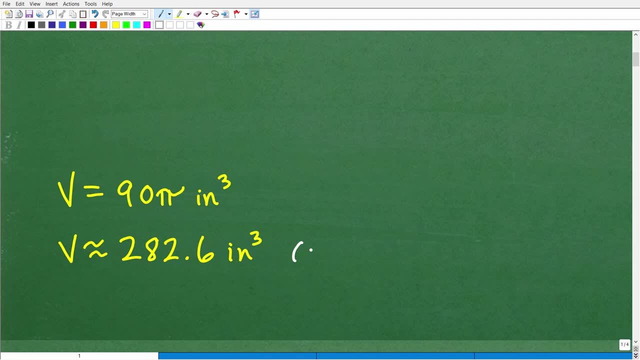 here I have these squiggly things. This is approximately, right, So this is approximately, which means it's an estimate, And this is exact. Okay, there is a difference. So the volume of the cylinder, the exact volume, is 90 pi inches cubed. Make sure you put in those units of measure. If you just put in 90 pi, for example, and you said, Oh, I got this right, Well, some mean math teachers would be like, Hmm, you didn't put in the units of measure. 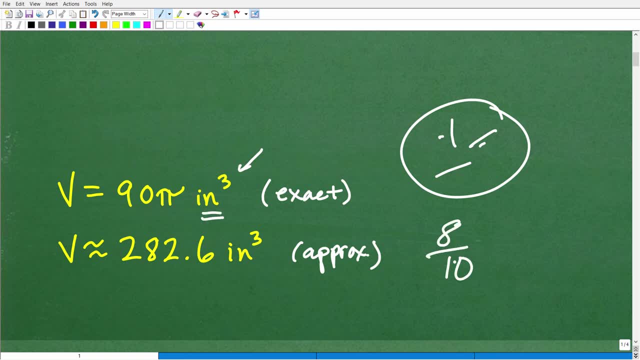 So I'm going to give you eight out of 10 points And you will not like that. You need to. anytime you're asked to do a area problem, surface area problem, volume problem, you need to put in those final units of measure. Anyways, units of measure here are inches, cubed, because our dimensions were in inches And you could use your calculator to get some sort of approximation. So for pi, for example, if you replace that with 3.14, well, pi is approximately 3.14. 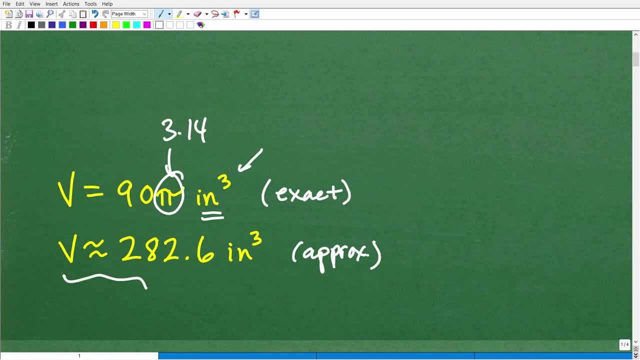 That's really a rough approximation, So the volume would be approximately roughly 282.6 inches cubed. But anyways, I will accept either one of these answers and give you full credit, And if you got either one of those, let's go ahead and celebrate with a nice little happy face. Oh, that's a terrible face. We could fix it up And a plus, a 100% and multiple stars, So you can show off to your friends and family that you know how to find the volume of cylinder. Okay, so good job. 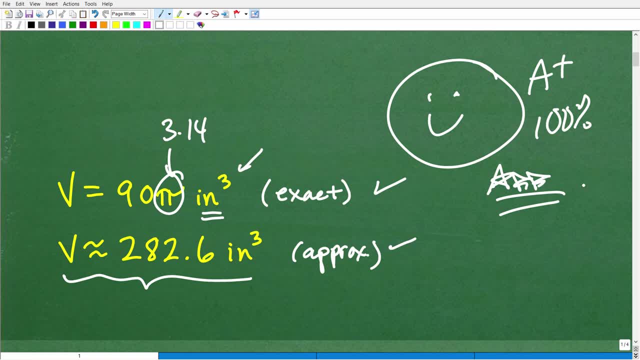 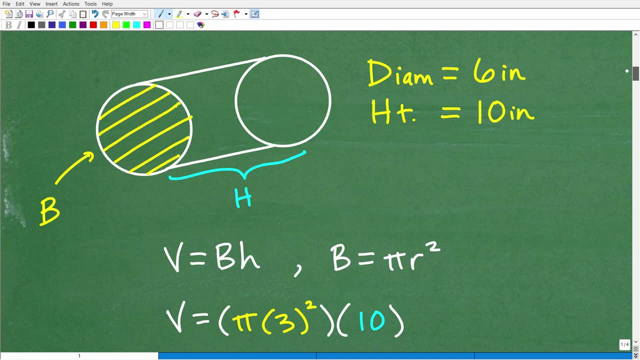 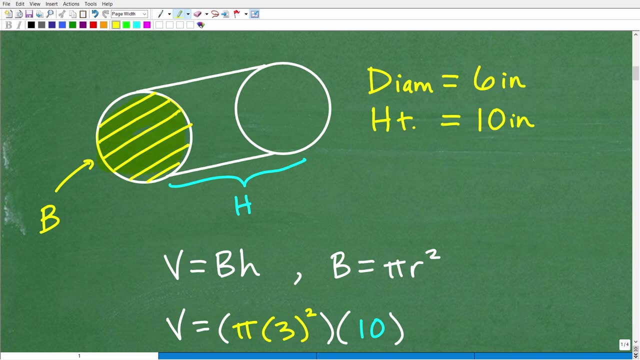 But again, what do you need to know to do this problem? You need to know the formula, Okay. so if you forgot the formula, let's go ahead and take a look at that right now. Okay so, the volume of a cylinder- pretty straightforward stuff. What you need to do is to find the area of the base. So we're dealing with a circle here, right? So we need to find the area of the base, ie the area of a circle. What's the area of a circle? Well, that's pi r squared, And that's another formula. Hopefully you remember that. 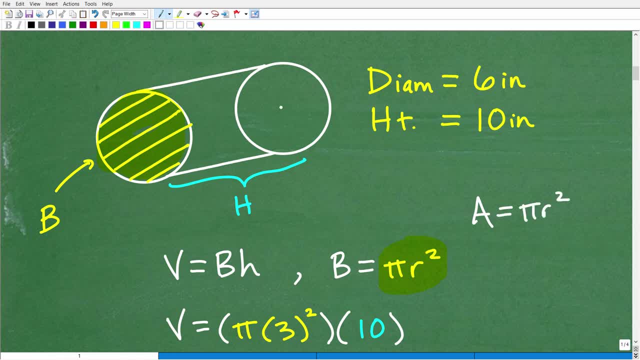 So the area of a circle is pi r squared, where r is the radius. So here we're, given the diameter, It's being six inches. The radius is half of the diameter. emanates from the center of the circle, So it would be one half the diameter. So in this case it's going to be what? three inches? Okay, All right, So that's what the B is. So the volume, matter of fact, I should just kind of tell you the formula Boy. I tell you- I was kind of getting ahead of myself here- Volume is base times height. All right, That is the volume of a cylinder. 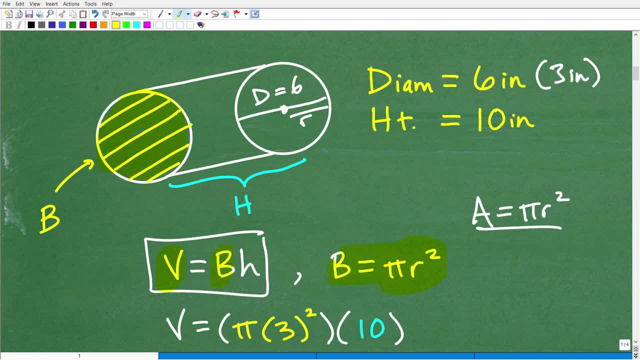 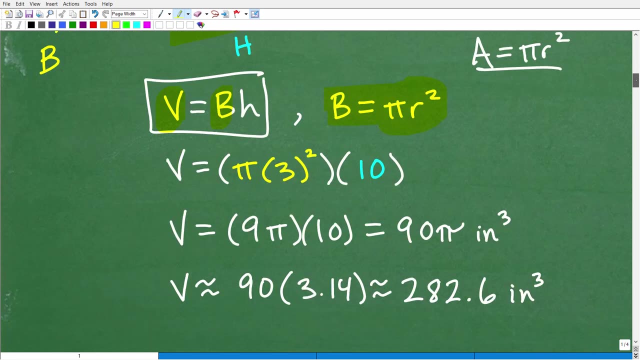 Volume is base times height. So B again is the area of the end- Okay, One of the ends of the cylinder. All right, So that's that. And then the height is obviously like the length of the cylinder. In this case it's 10 inches. All right, So pretty straightforward stuff. So let's go ahead and calculate right now. All right, So the volume is going to be equal to the area of the base, which is pi r squared. 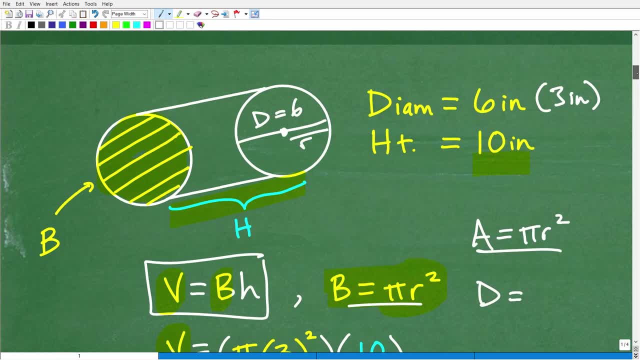 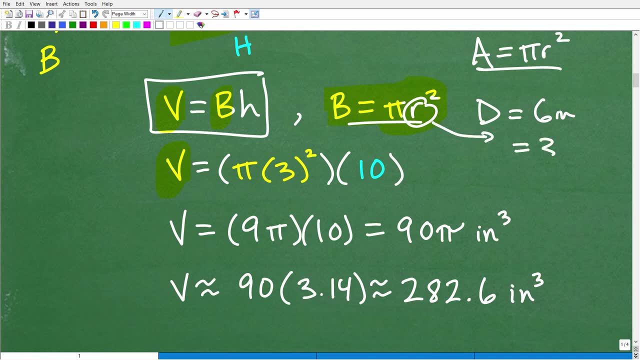 Now remember the diameter where we're given being six inches. Okay, Well, we don't need the diameter, We need the radius. That's going to be one half of the diameter, So that'd be three inches. So it's going to be pi. r squared, So r is three, So three squared times pi. This, right here, is the area of the base of three. squared is what. three times three is nine, So this is nine. pi Ten is our height, Right? So we remember, right here. 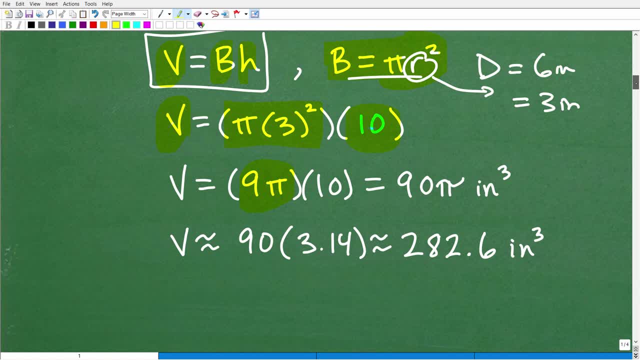 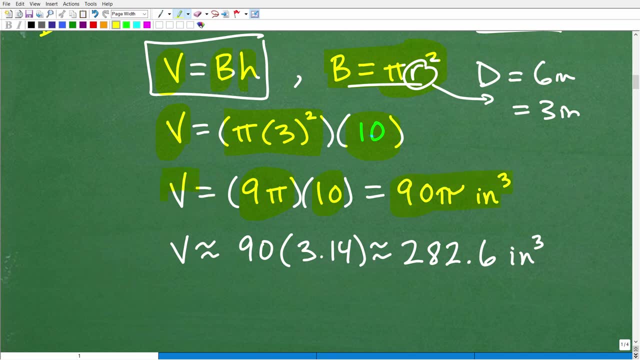 We were told that the height of the cylinder or the length of the cylinder is 10.. So we have nine times pi times 10.. Nine times 10 is 90. So 90 pi. So if you're asked- and it's very important that you know the language in terms of these questions- So if the question is find the exact volume of this cylinder, this would be the exact volume. So just leave your answer with pi. That's perfectly acceptable And it is the most correct answer. 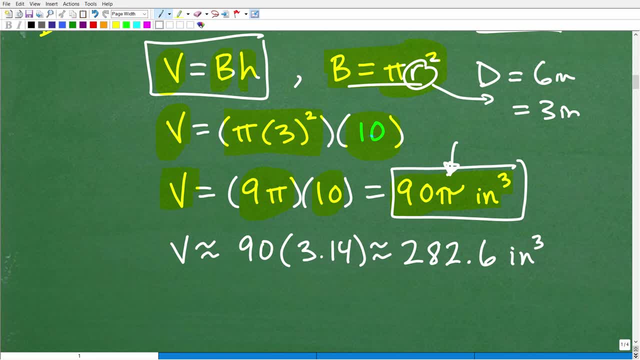 Okay. Now if you're asked to find the approximate volume of a cylinder or to give it a decimal approximation, that's when you can go ahead and substitute in for pi and approximation And you can get various levels of more accurate estimations of pi by using your calculator. Okay, But the most basic decimal approximation of pi is 3.14.. So it's 90 times 3.14.. And you're going to approximately 282.6 inches cubed. 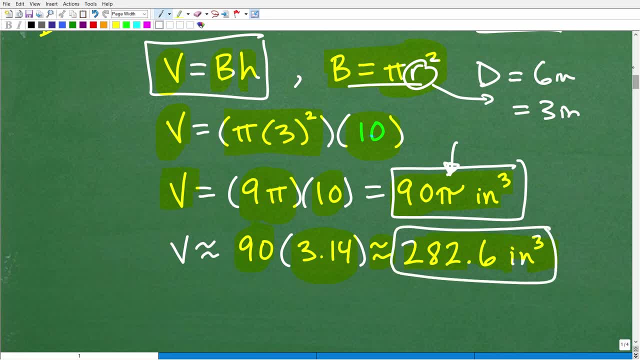 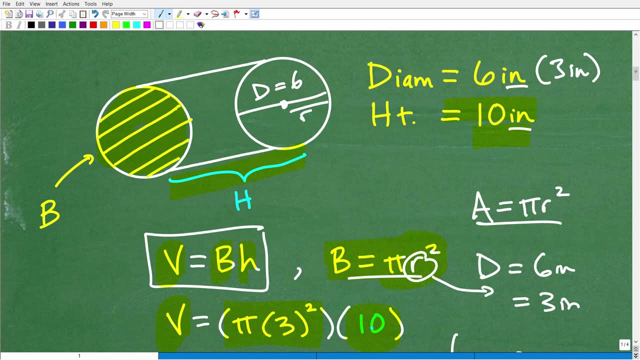 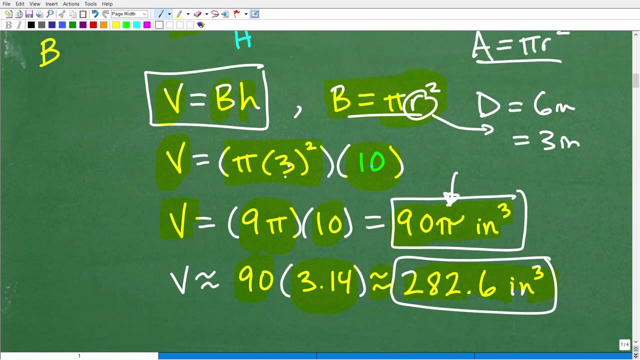 Again, we're dealing with inches, All right. So remember, our diameter is in inches, Our height is in inches And this volume is going to be in inches cubed. Okay, So, just so you understand what's going on right here, we're taking the radius and we're squaring it. Okay, So the radius is in inches, So we're going to end up with inches squared right there And then we're going to multiply by inches. Again, this would be height, So we get inches squared times inches, So we end up with inches squared.